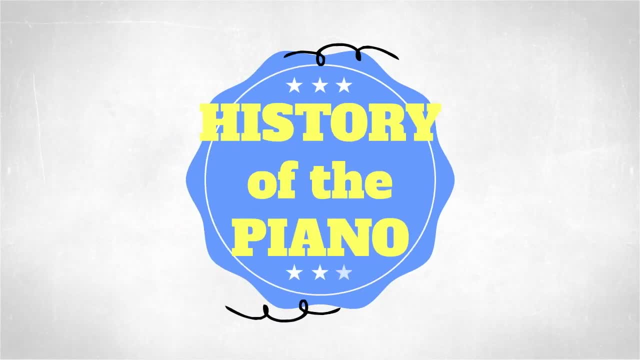 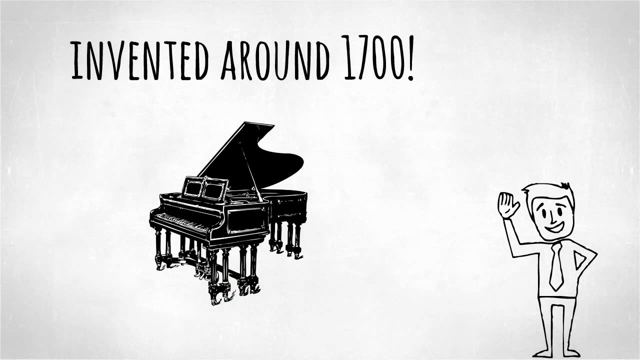 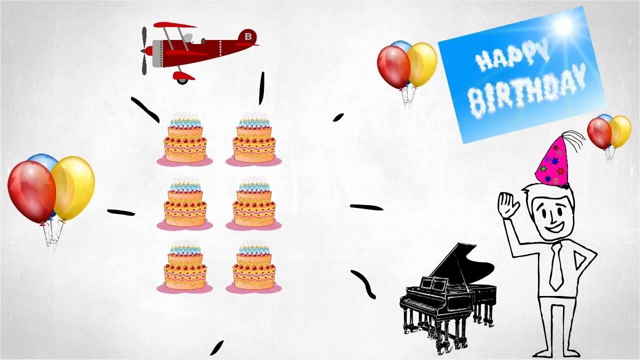 The history of the piano. The piano has been around for a long time. Although we do not have an exact date, we know that the piano was invented around the year 1700. That is, over 300 years ago. Gee whiz, that would be a lot of birthday cakes and candles to celebrate the piano's birthday every year. 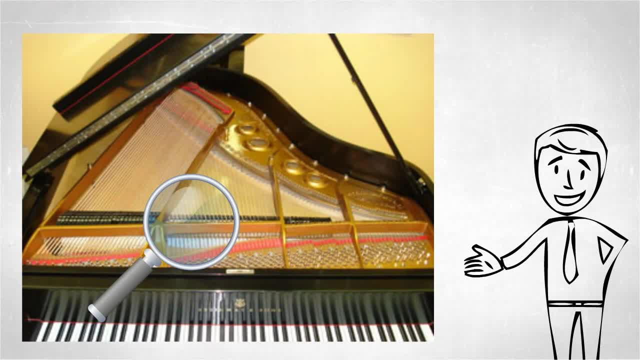 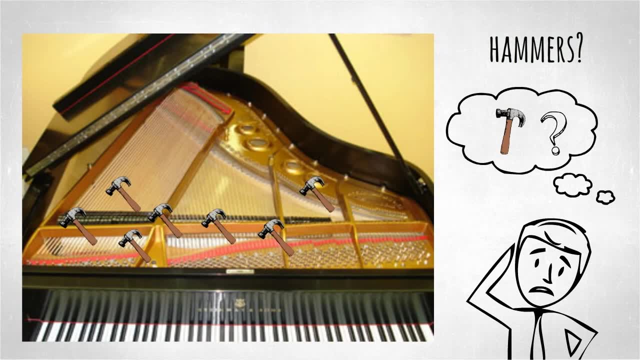 Okay, let's take a closer look inside the piano, because that is the part that gives the piano its great sound. Inside the piano, we have hammers- Now wait a second, not those type of hammers. If we use those hammers, our poor piano would most likely be broken. 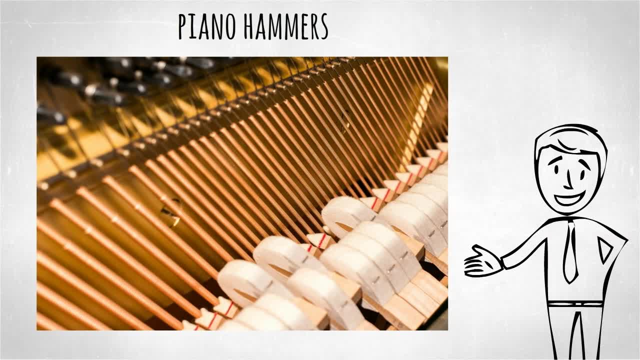 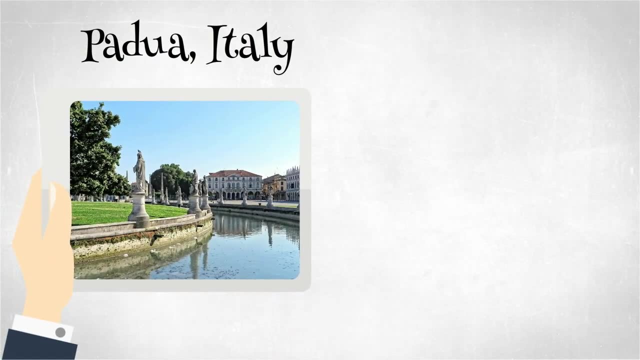 I'm talking about the piano hammers. Piano hammers have a felt covering, as you see here. When we press a key down on your piano, the piano hammers hit the string which creates a beautiful sound on the piano. A long time ago in Padua, Italy, a man named Bartolomeo Cristofori was eating delicious pizza With pepperoni. 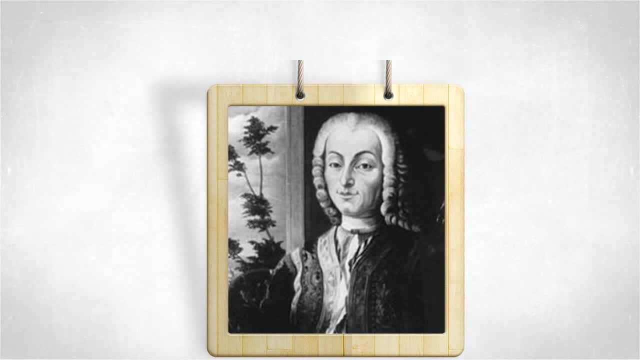 Okay, Cristofori was doing more than just eating pizza. He was the guy who invented the piano. He thought to himself: I wonder if I could make an instrument that was better than the harpsichord. But then he was quickly distracted by that pepperoni pizza. 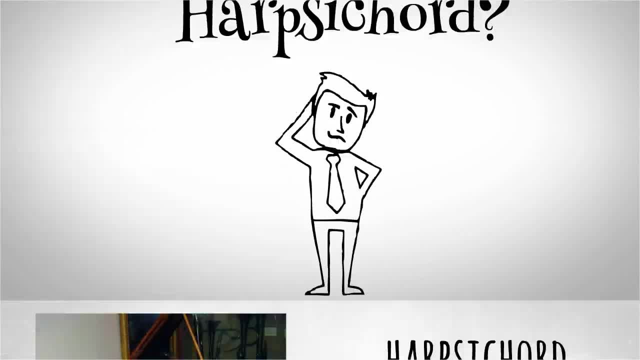 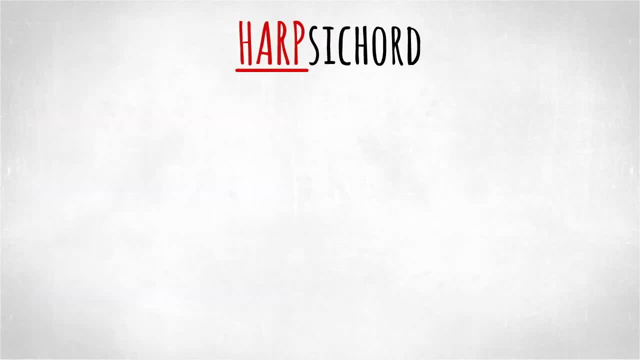 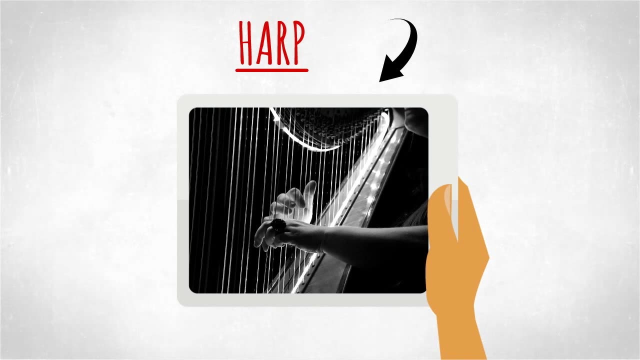 Harpsichord. What is that? The harpsichord is an instrument that was invented before the piano. It looks a lot like a piano, but it works differently. In the word harpsichord we have the word harp. A harp, when played correctly, is plucked by the fingers to create the sound. 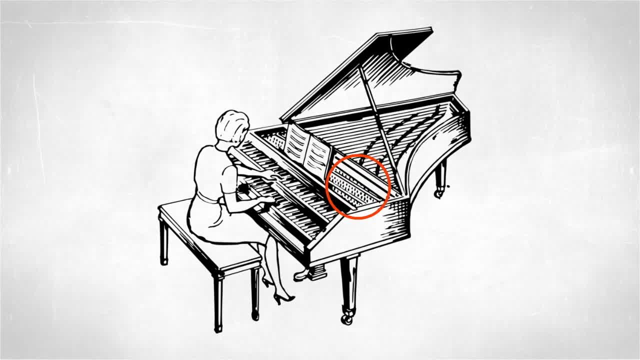 When a person plays the keys on the harpsichord, the strings are plucked by a small quill, not struck with hammers. Since the strings are plucked by small quills, the volume is always higher. The harpsichord is the same. You cannot play loud or soft on the harpsichord. 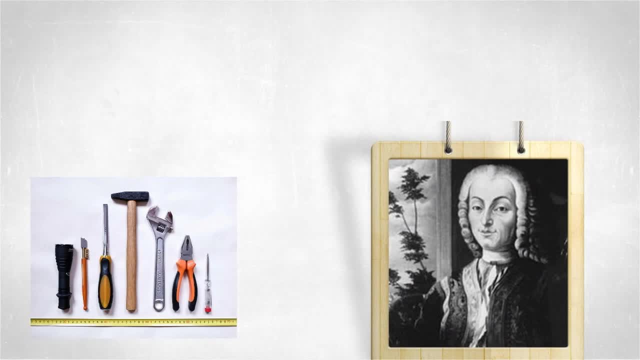 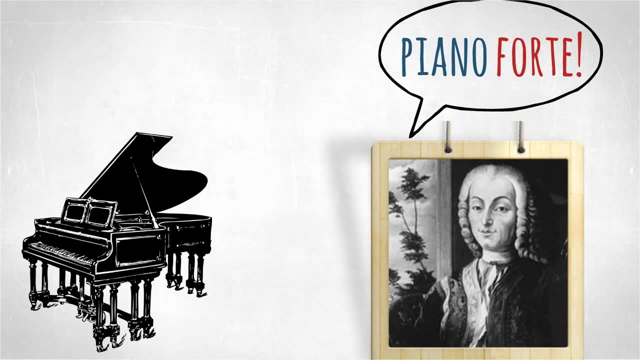 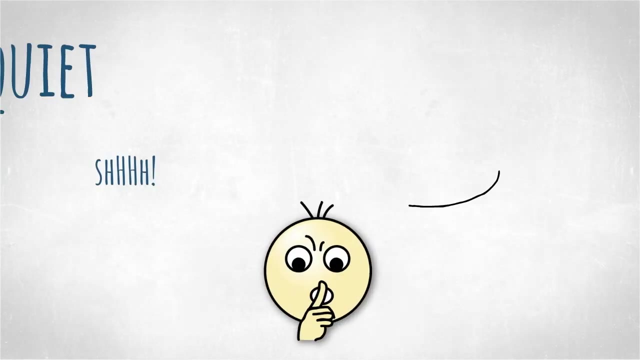 Cristofori was working hard building his invention. He actually made 20 of them and originally called it the pianoforte. Let's take a closer look as to why he called it the pianoforte. In Italy they speak Italian and the word piano means quiet.